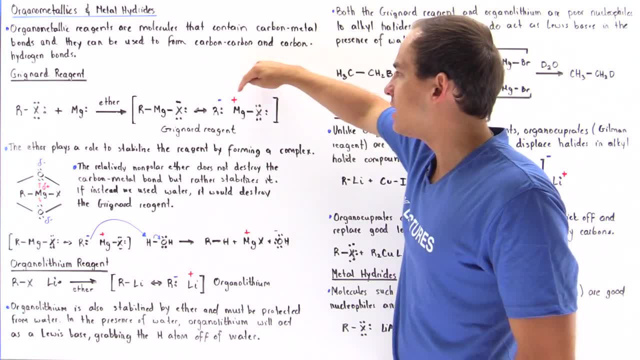 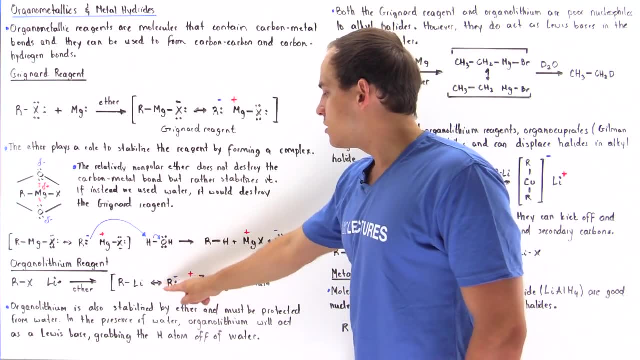 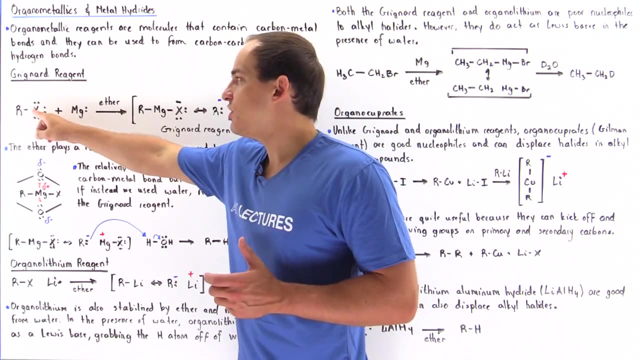 the magnesium. this carbon pulls away those electrons and this bears a negative charge. this bears a positive charge. Likewise, in this case, this bears a negative charge, this bears a positive charge. Now, why is it that we cannot use a fluoride for our halogen? Well, fluoride is the most electronegative. 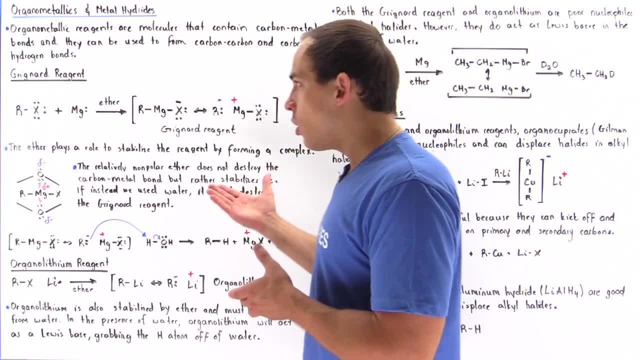 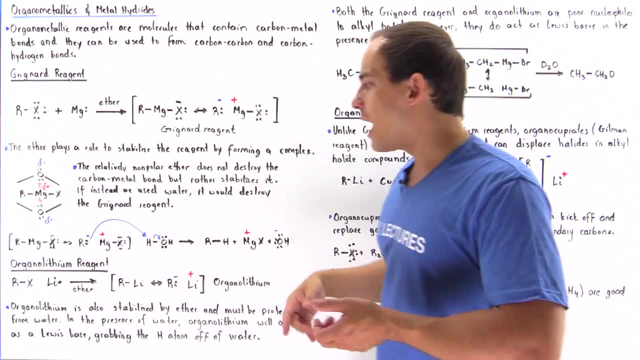 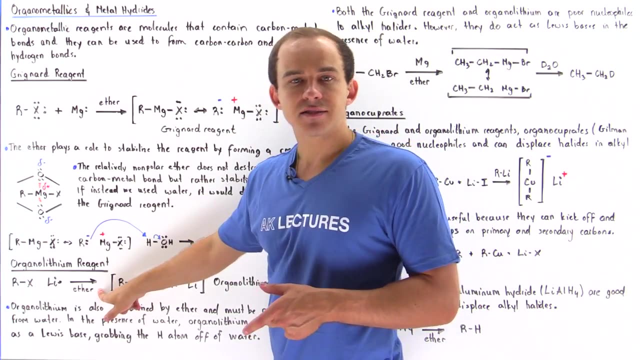 atom and it forms a very strong bond. So with fluoride this reaction will not take place. But if we use our iodide chloride or bromide, this reaction will take place. Now the second question is: why do we have to use ether as the solvent? Well, ether is relatively nonpolar, and ether 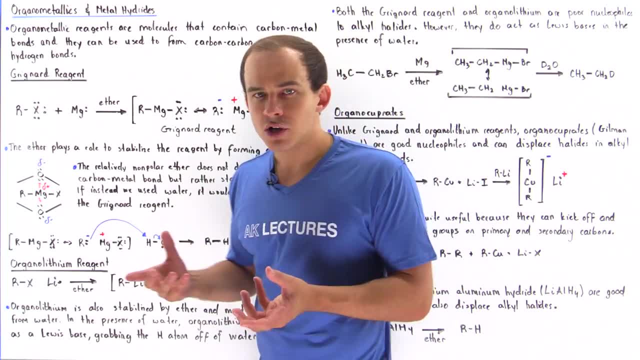 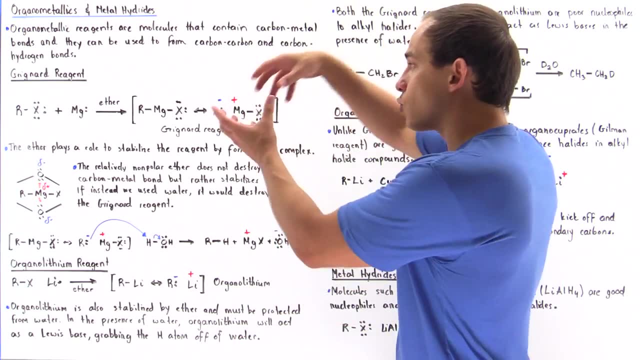 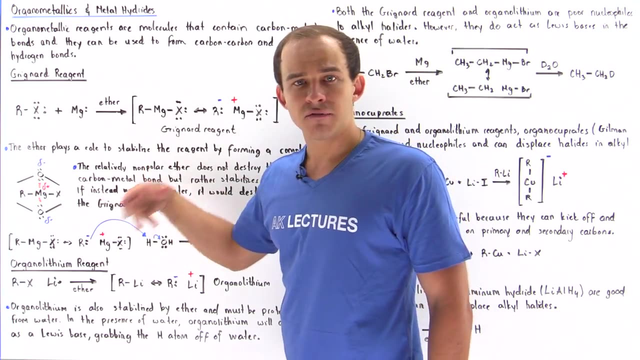 basically creates a very stabilizing structure with our Grignard reagent as well as the organolithium reagent. The ether basically surrounds these two reagents and forms stabilizing interaction between the oxygen of the ether and our metal atom. So for the case of our Grignard reagent, the magnesium- 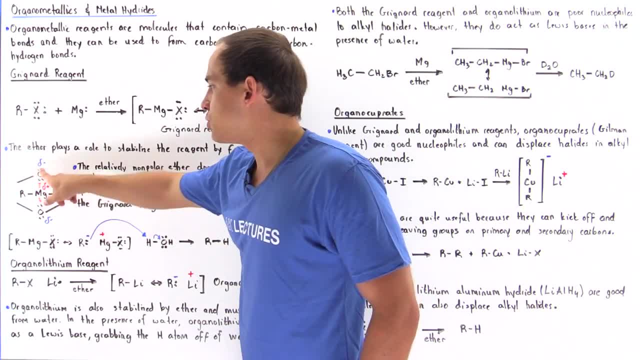 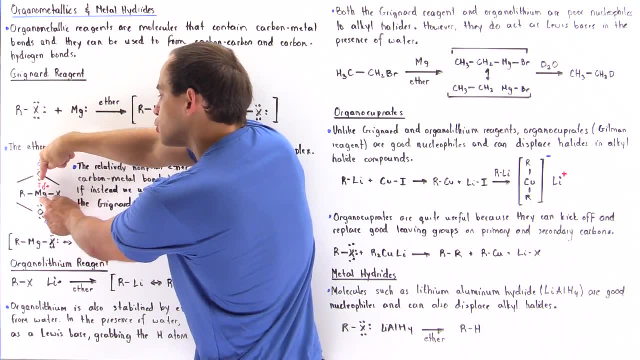 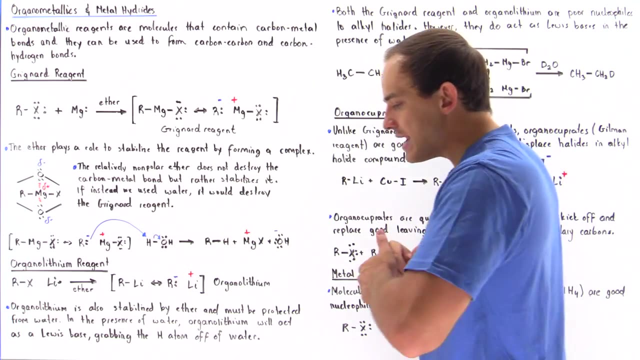 has a partial positive charge. These oxygens will have a partial negative charge and so they will surround and form stabilizing interactions shown in orange, and this will stabilize these organometallic reagents. Now, what are these reagents actually used for? Well, 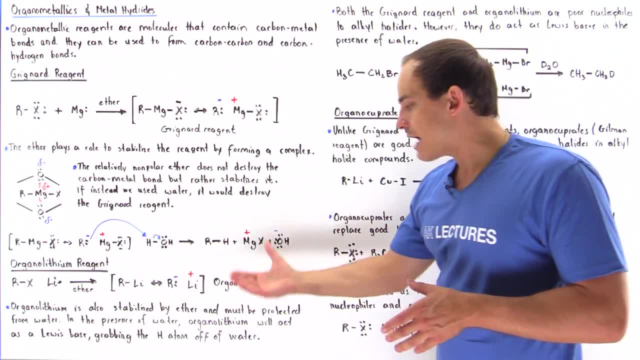 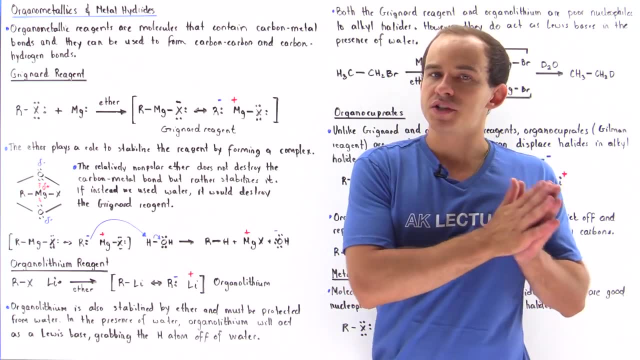 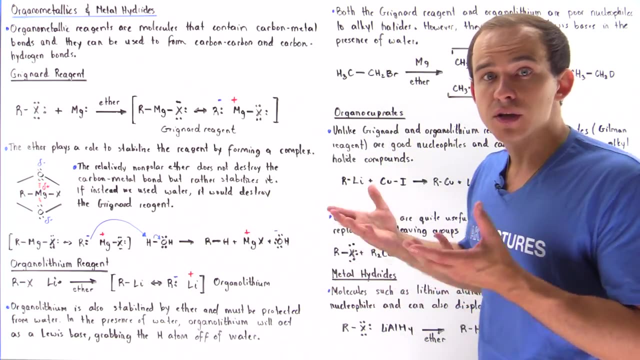 if we take either the Grignard reagent or the organolithium reagent and we mix it in the presence of water, the Grignard reagent will act as the Lewis base, while the water will act as the Lewis acid, will have a Lewis acid base reaction to produce a bond between carbon and hydrogen. So if we examine 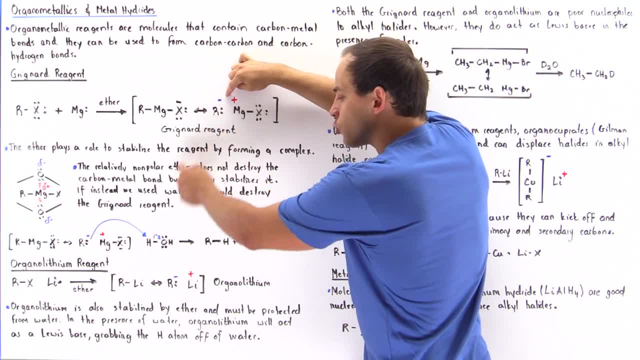 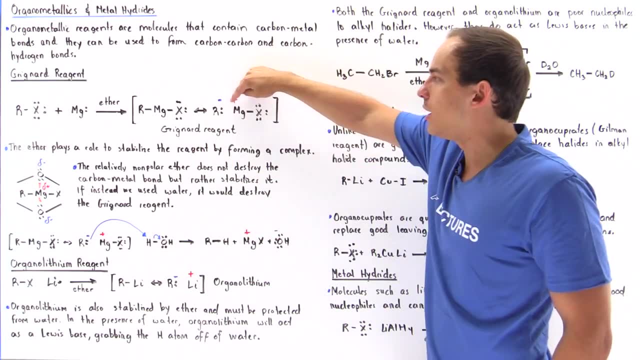 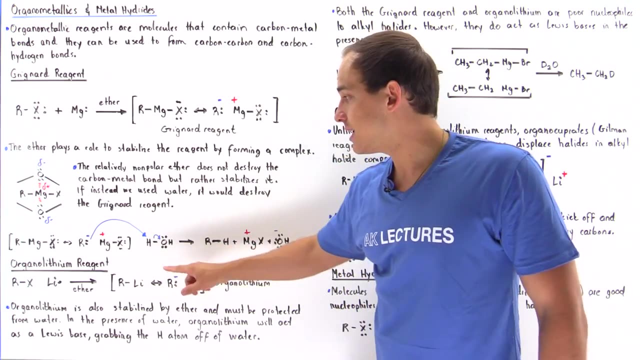 this resonance stabilized structure. the R groups bear a full negative charge because the carbon contains those lone pair of electrons And this can act as a Lewis base. in the presence of water, The water acts as the Lewis acid and these electrons take the H atom away from water. 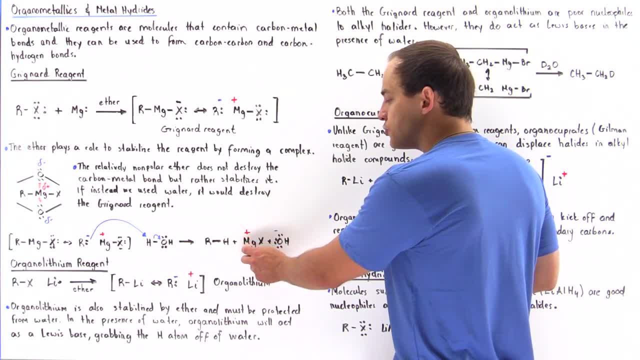 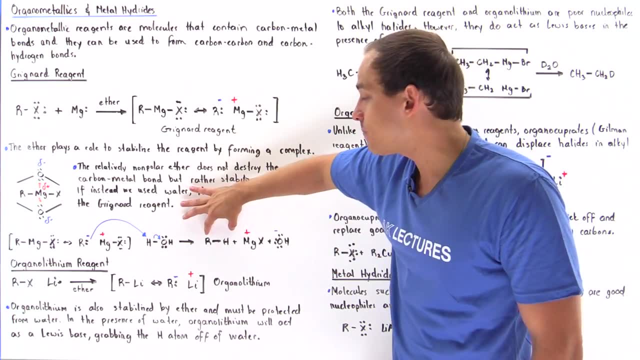 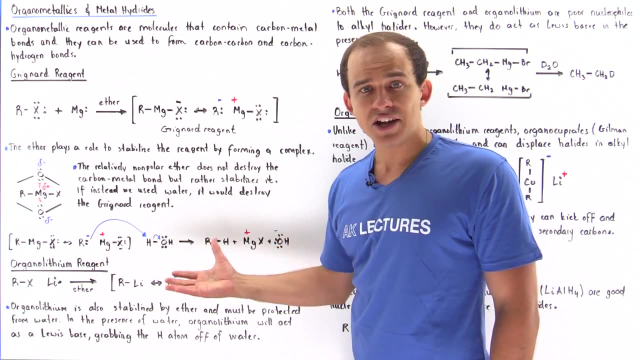 to form the hydroxide, the MgX, where Mg has a positive charge, and the bond between carbon on the R group and our H. So we form the carbon-H bond. So by using the Grignard reagent or the organolithium reagent, we essentially form carbon-hydrogen bonds. 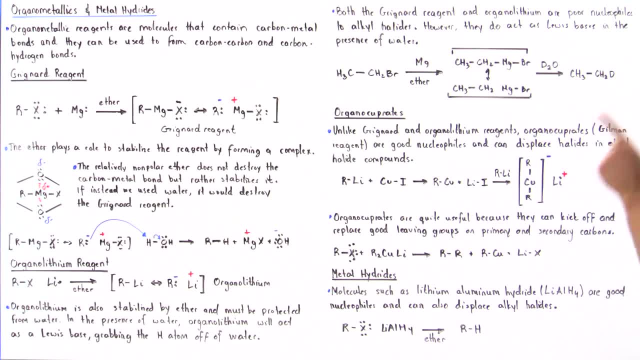 So both the Grignard reagent and organolithium reagents, although they are good enough Lewis bases to react with water, they are not very good nucleophiles and will not displace good leaving groups on alkyl halides. So now, if we take for example the following molecule: 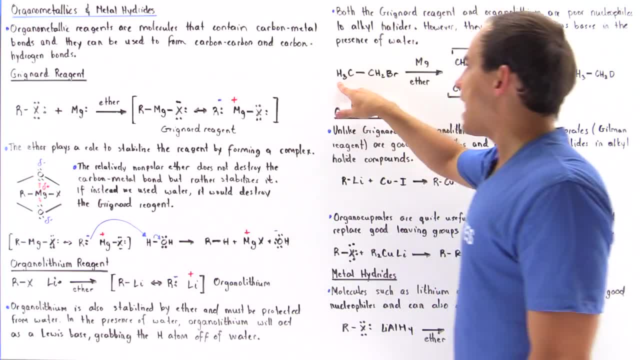 one specific example in which the R group is the ethyl group and our X is the bromide. So if we take, for example, the following molecule, one specific example in which the R group is the ethyl halides. So if we take, for example, the following molecule, one specific example in which the 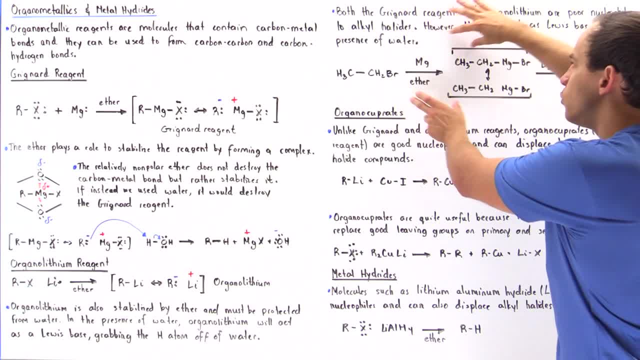 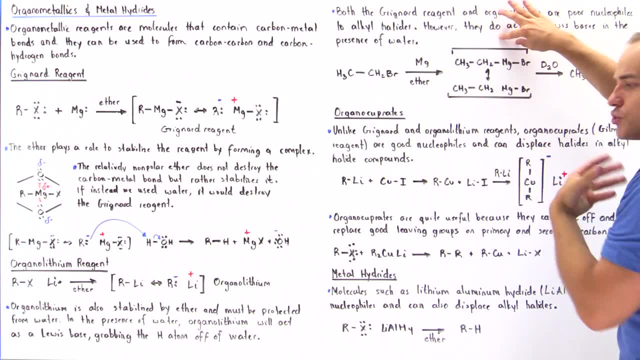 bromide and we mix it with Mg ether, we produce this resin-stabilized structure. Now we can also mix it with lithium to produce our organolithium reagent. And if we mix it with water in which the H atom has been replaced with deuterium, our radioactive atom, we produce the following: 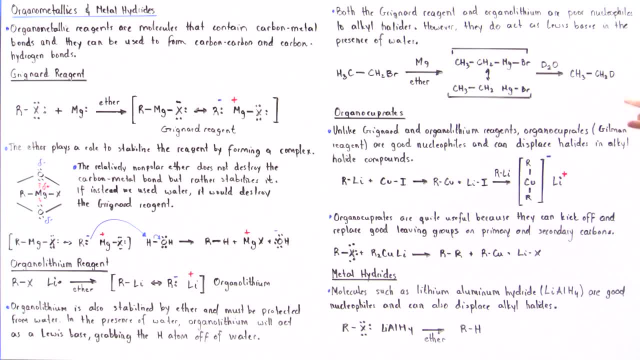 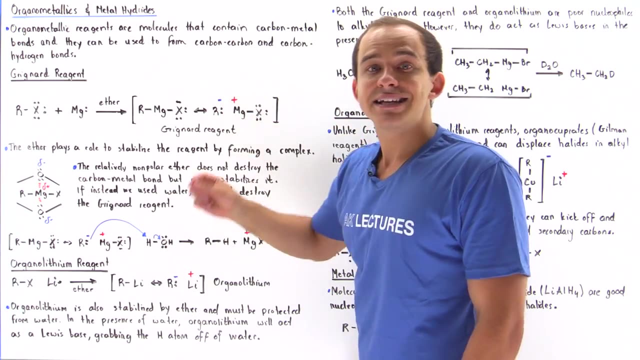 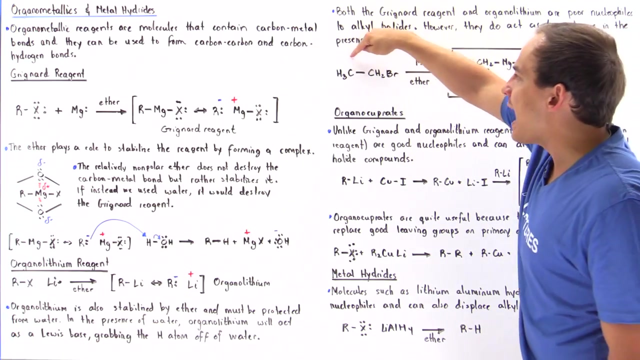 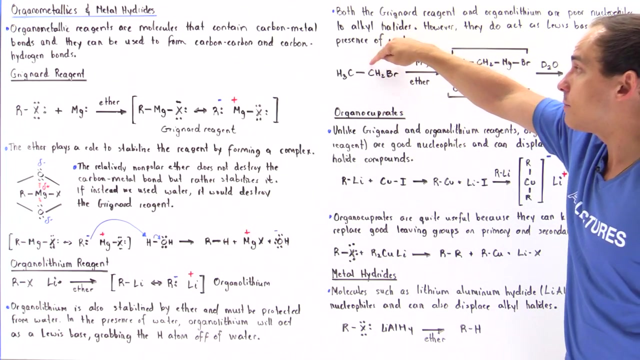 product in which the bromide has been replaced with our deuterium. So we form a bond between carbon and our deuterium. Notice that this atom, or this actually molecule, the R with our two electrons, is not a good enough nucleophile to actually displace this bromide and attach and form a bond between the carbon on this R group and a carbon on this and the carbon on this molecule. However, other organometallic reagents 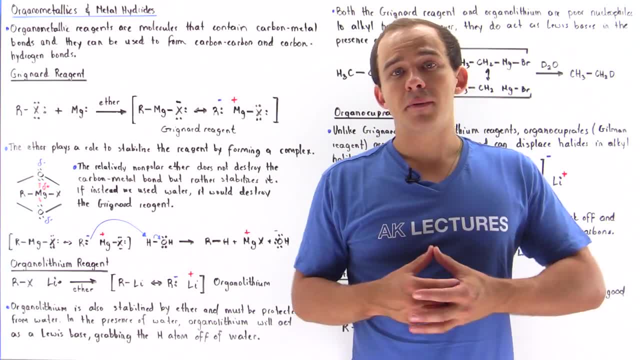 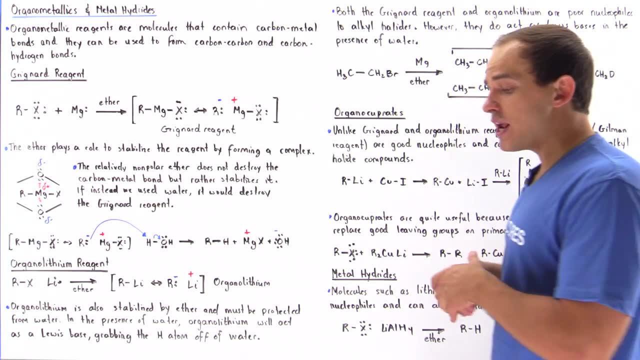 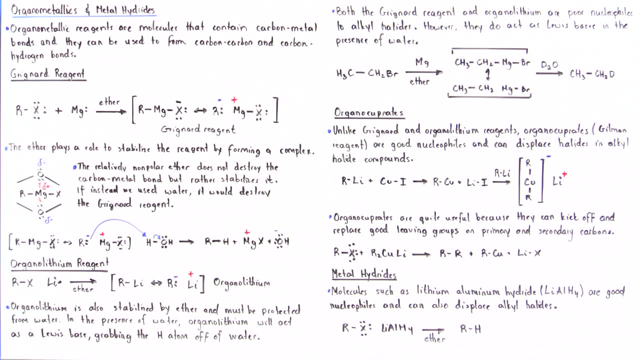 do exist that do form carbon-carbon bonds, because they do have a good enough nucleophilicity, And such organometallic reagents are known as organocuprates. So, unlike Grignard and organolithium reagents, organocuprates, also known as Gilman reagent, are good nucleophiles and can displace halides in alkyl halide compounds. So let's begin by 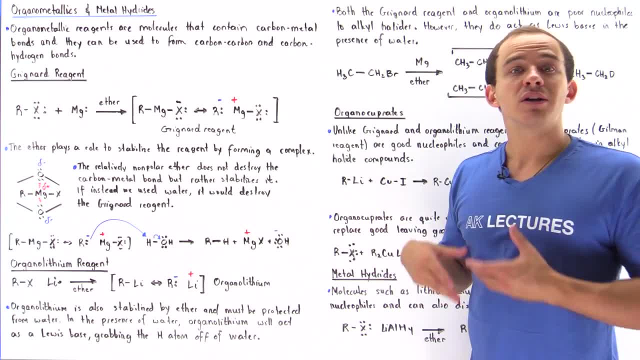 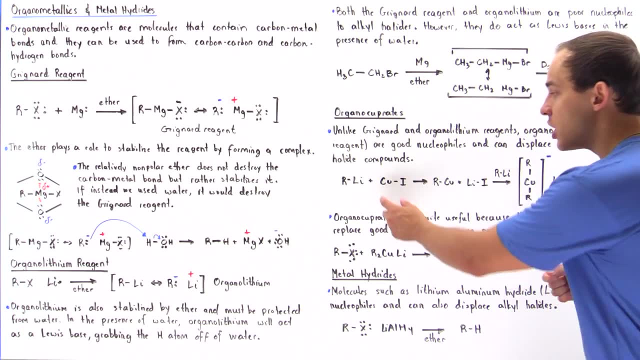 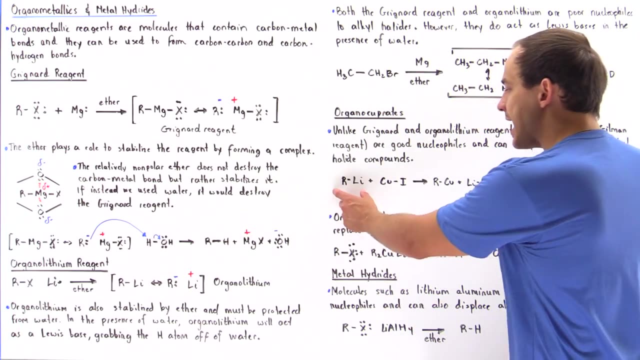 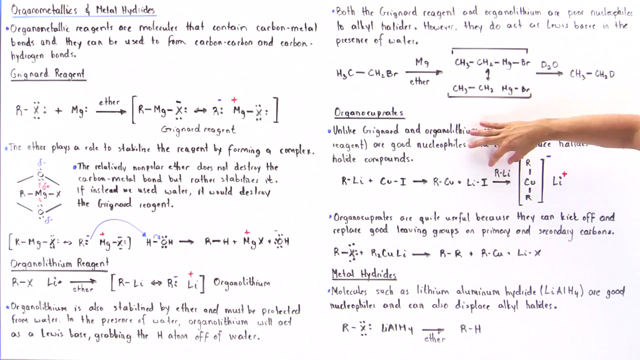 discussing the R group. So let's begin by discussing how we can actually form our lithium organocuprate, one type of organocuprate. So basically, we have to mix copper iodide with our RLi, where this is our organolithium reagent. If we mix these two, we produce this, And then, if we mix it once again with our organolithium reagent, we produce the lithium organocuprate. that looks like this: 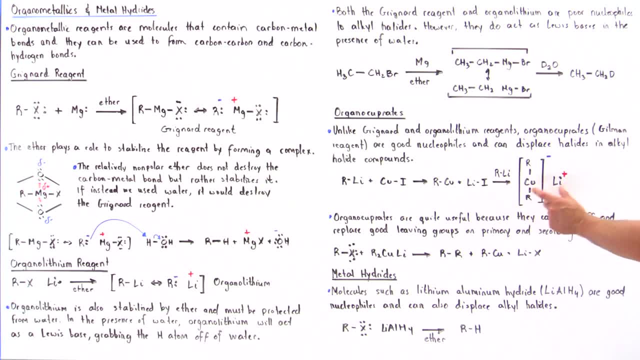 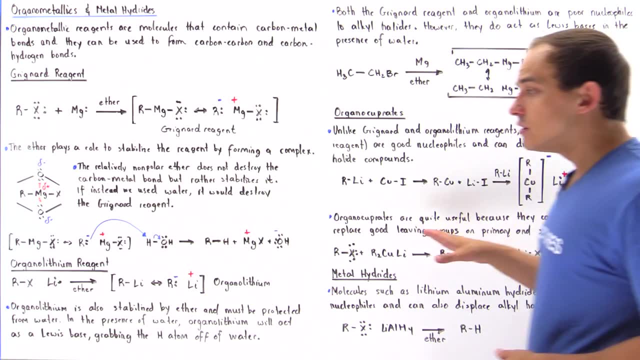 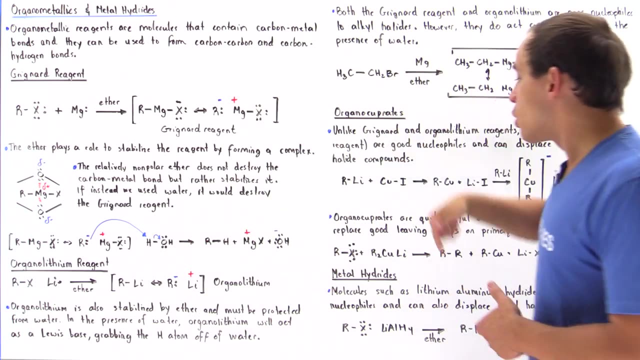 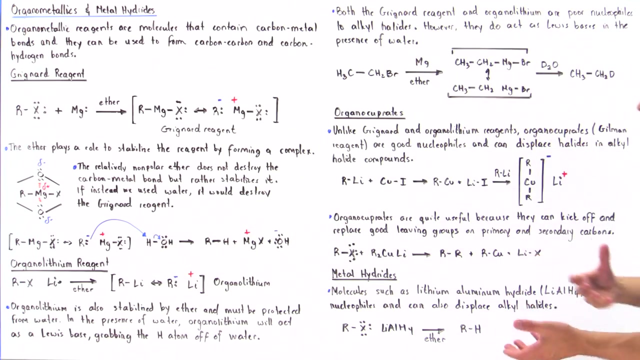 this. so we have a positive charge on the lithium, a negative charge on this molecule and they bond via electrostatic forces. so, unlike organolithium reagents and our Grignard reagents, which are poor nucleophiles, organocuprates are quite useful because they are good enough nucleophiles to basically displace and 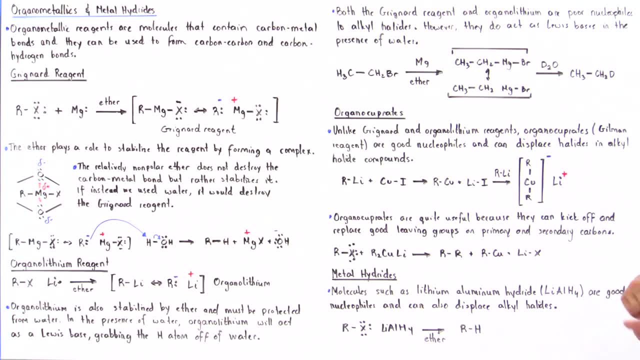 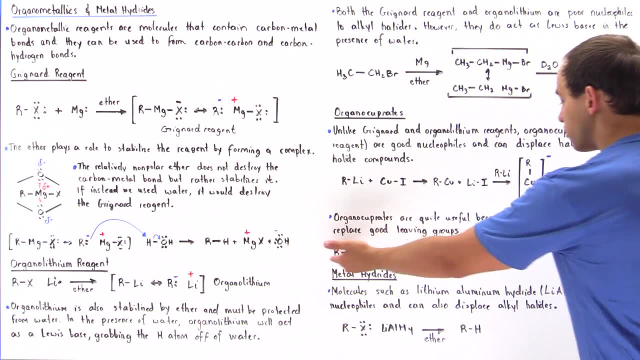 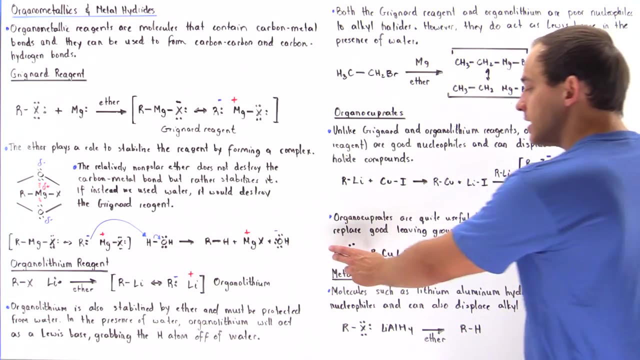 replace good leaving groups on primary and secondary carbons and one particular example or the general. the general example for this reaction looks something like this: so we have our primary or secondary hydrocarbon that contains the good leaving group, or X is our halogen that could be chloride. 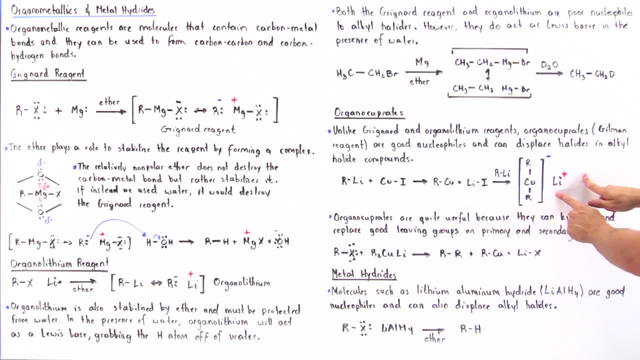 bromide or iodide, we mix it with the lithium organocuprate and we produce or or or or a bond between the carbon on this atom and a carbon, or a carbon on this group and a carbon on this R group. So we form the following carbon-carbon bond and we form this structure. 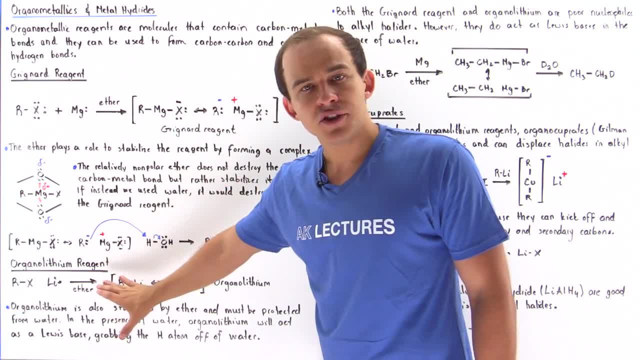 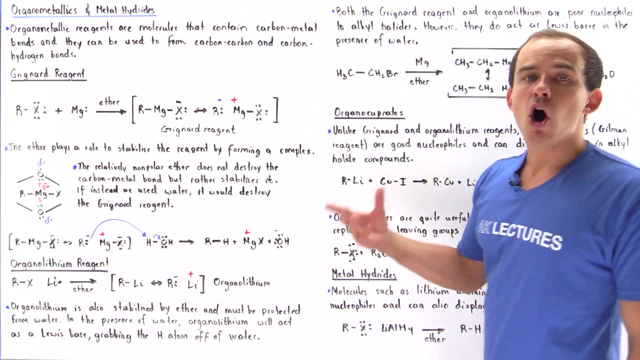 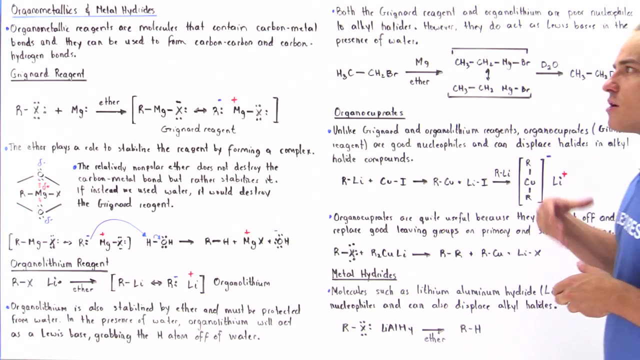 here. So Grignard reagent and organolithium reagent are used to form carbon-hydrogen bonds, but organocuprates are used to form carbon-carbon bonds. Now, finally, the final thing I want to briefly talk about are metal hydrides. So metal hydrides are basically complexes. 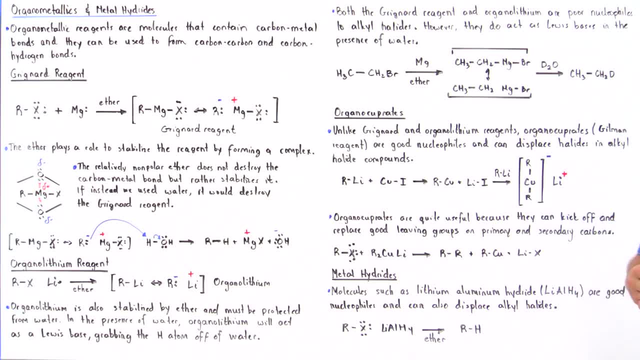 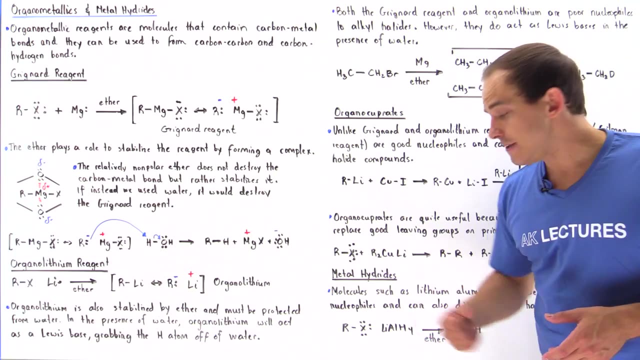 that can be used as nucleophiles to replace our good leaving groups on organic halides. So if we, for example, take the following: Rx, where R is our organic compound and X is our good leaving group, and we mix it with one type of metal hydride- lithium, aluminum hydride-